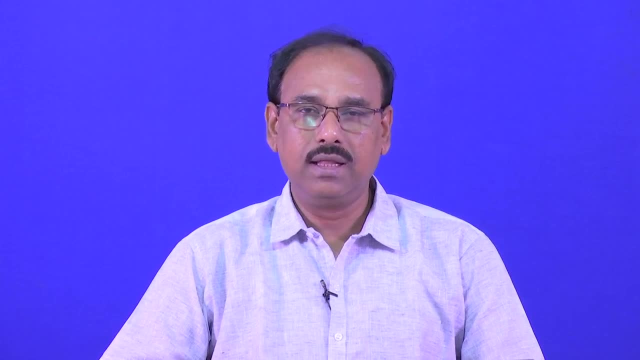 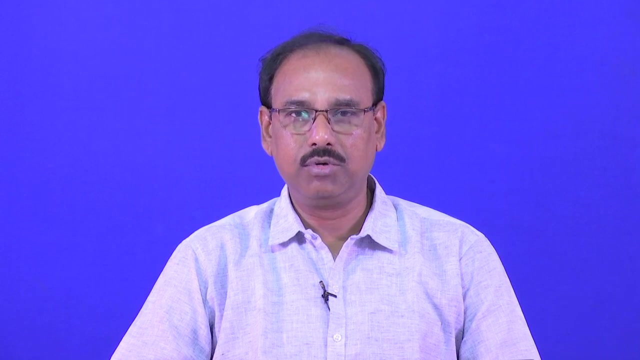 having a lesser number of nodes than the input layer, the network learns a compressed domain representation. What will happen if the hidden layer contains the same number of nodes as the input layer, or the number of nodes which is even larger than the input layer? Later on, of course, we will see other configurations. 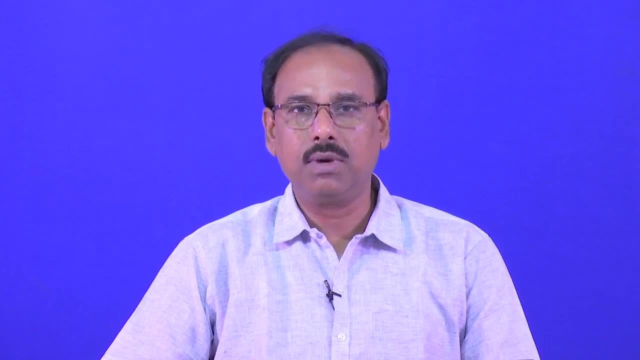 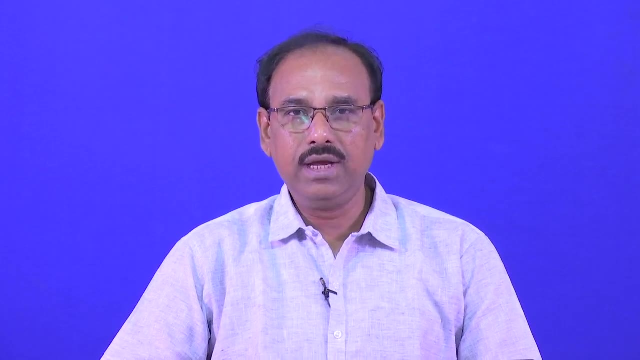 Of the autoencoder, where such thing is also possible. but in such cases the autoencoder will learn a compressed domain representation by introducing some constant which we will term as sparsity constant. We will come to that later, but so far what we have discussed. 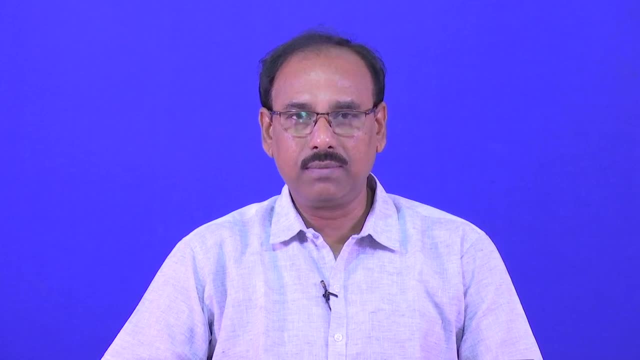 is what is known as under complete autoencoder. So there, if we assume that your number of nodes in the hidden layer is same as the number of nodes in the hidden layer, So the number of nodes in the input layer and obviously the same as number of nodes in the output. 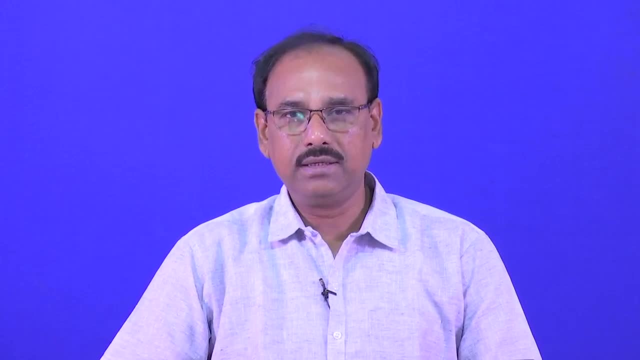 layer, and or even more than that. In that case, it is possible that autoencoder will simply try to memorize the input data, and the function that it will learn is a simply identity function, whereby wherever is there at the input, the same will be reproduced at. 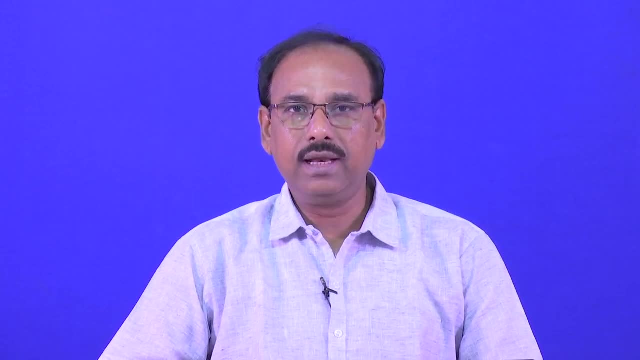 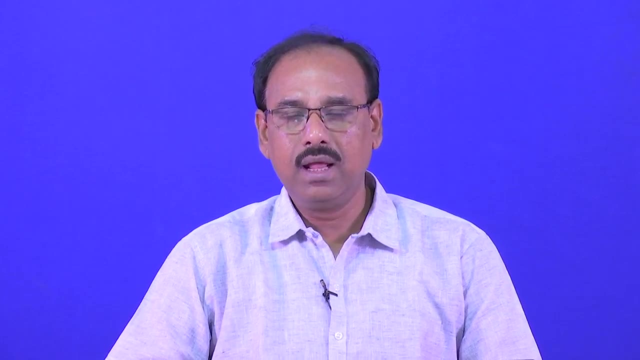 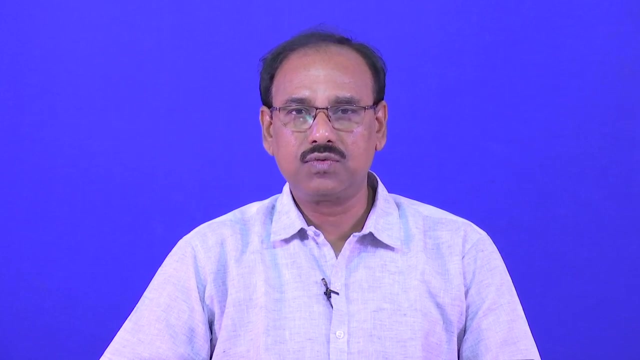 the output, But by putting a hidden layer having limited number of nodes, known as bottleneck layer, as we have just said, the network is forced to learn a compressed domain representation, or the network is forced to learn the salient features which are present in the input data, and that is the purpose of an autoencoder. 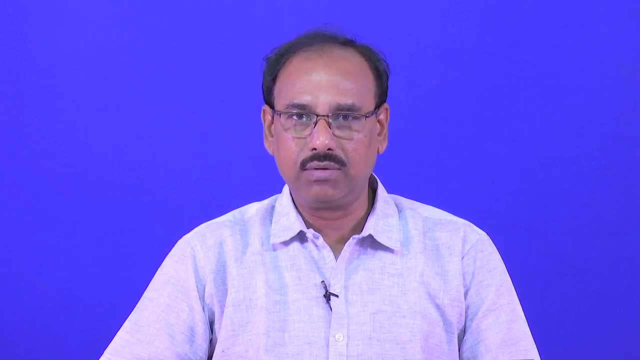 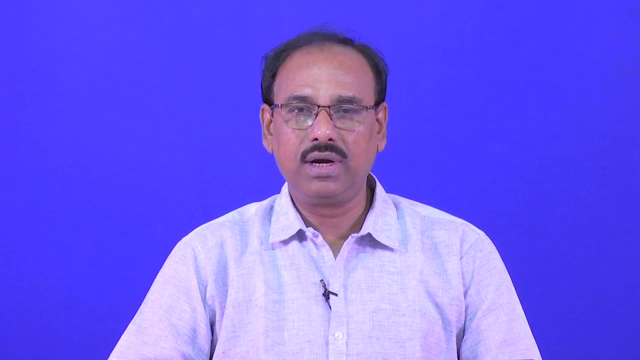 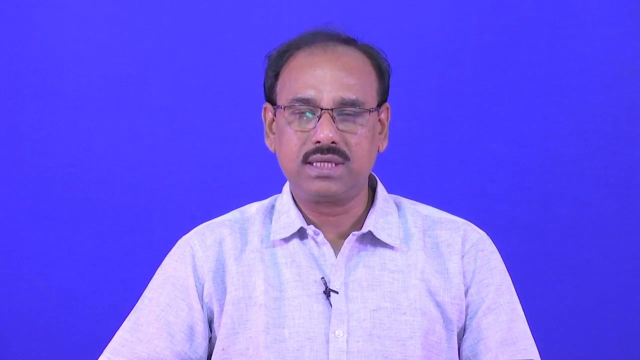 Reconstruction of the input signal is not the purpose of autoencoder. but the purpose of autoencoder is that it learns A compressed domain representation, or it learns the salient features in the input data and, using this salient features, the decoder side should be able to reconstruct your original. 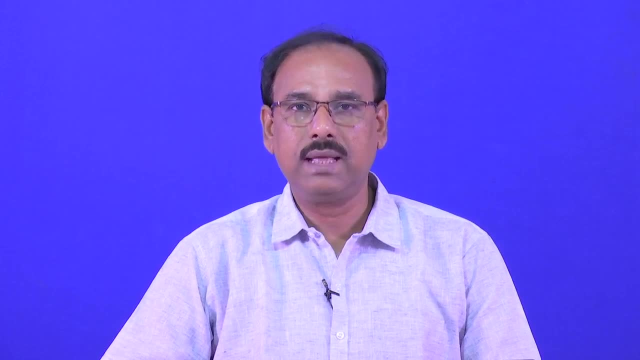 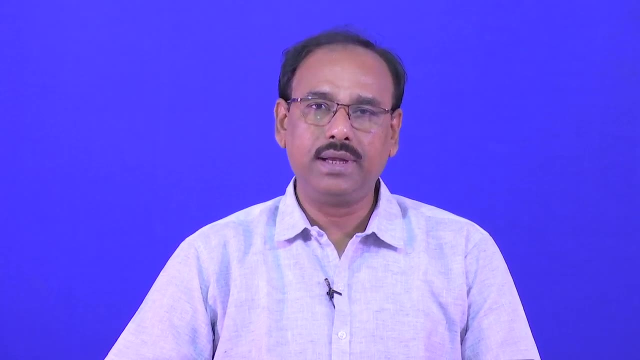 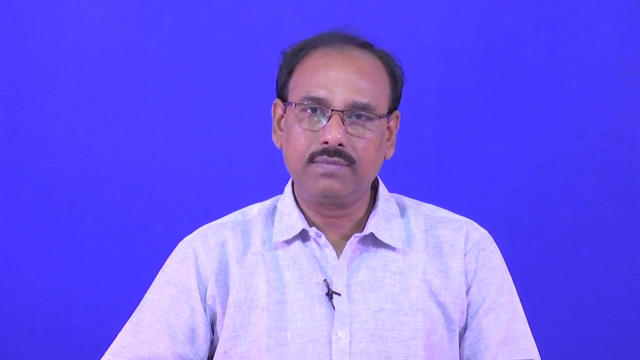 data. So we are actually interested when it comes to the application of autoencoder- we will come to that a bit later- we are actually interested in the output of the hidden layer, or the bottleneck layer, which is a compressed domain representation. Now we have also seen that, as we are talking about the compressed domain representation, 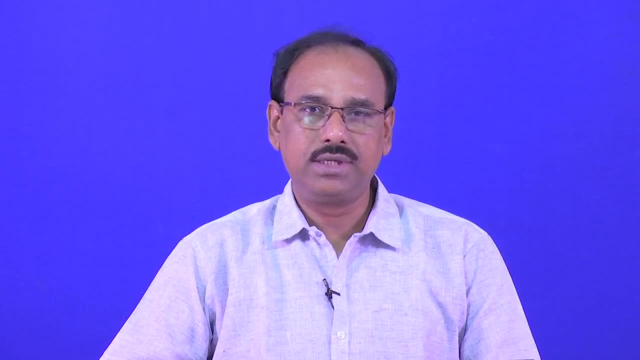 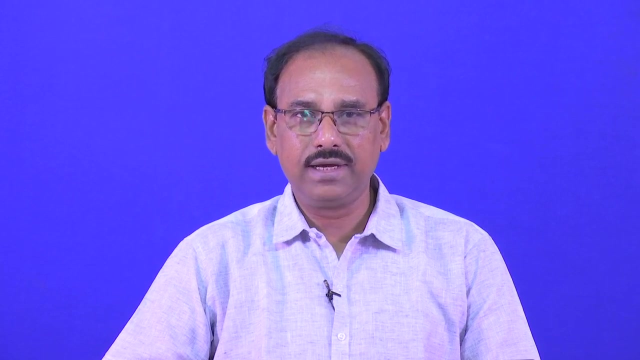 this is also nothing but what is known as dimensionality reduction. So if your number of nodes in the hidden layer is much less than the number of nodes in the input layer, then in the compressed domain representation the dimensionality of the latent variable. 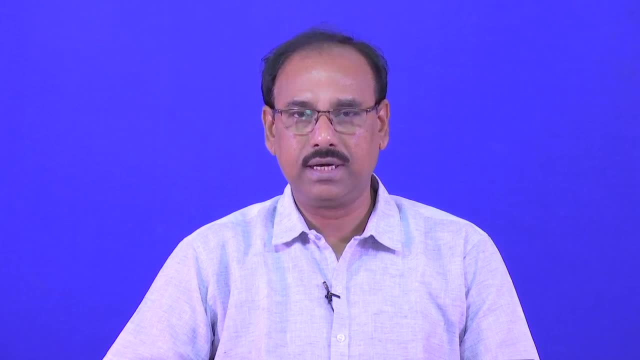 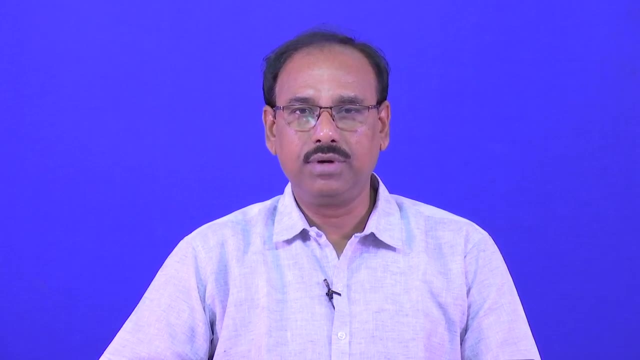 which is mapped from the input data. the dimensionality of the latent space data is much less than the dimensionality of the input data, But still the decoder should be able to reconstruct the input from that reduced data. So this is what is dimensionality reduction. 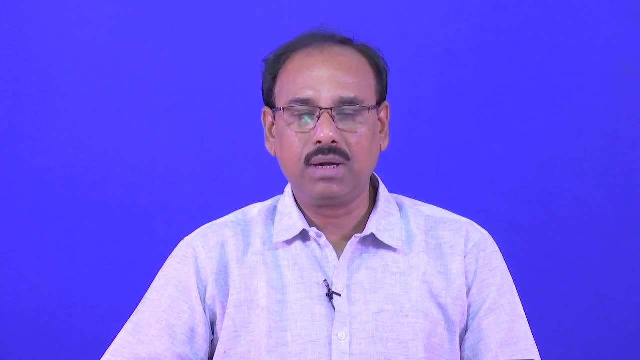 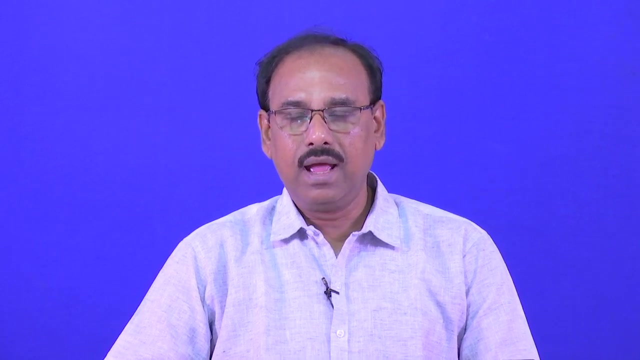 And we have also discussed in our previous lecture that when we talk about dimensionality reduction, traditionally a very popular method for dimensionality reduction is what is known as principal component analysis, That is, the input data isprojected in a way that it is projected onto the eigenvectors, into the eigen space. And if the input data is projected, 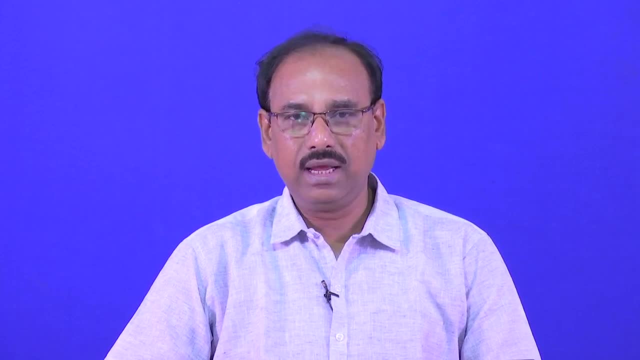 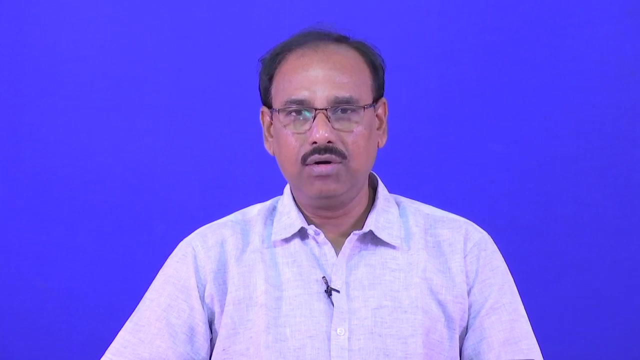 into the eigenvectors. obviously, if you haveset of data which is of dimension d, the number of eigenvectors will be d number of eigenvectors, but for every eigenvector there will be a corresponding eigenvalue. So when you form the transformation matrix, you form the transformation. 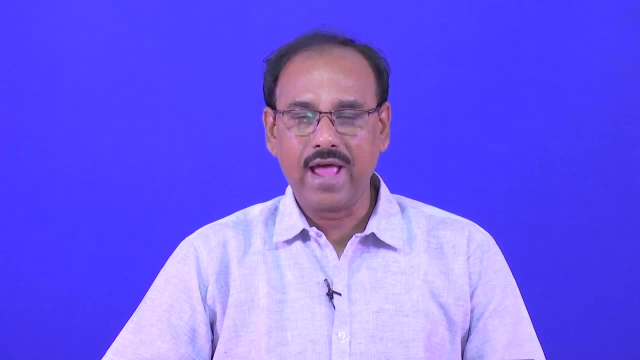 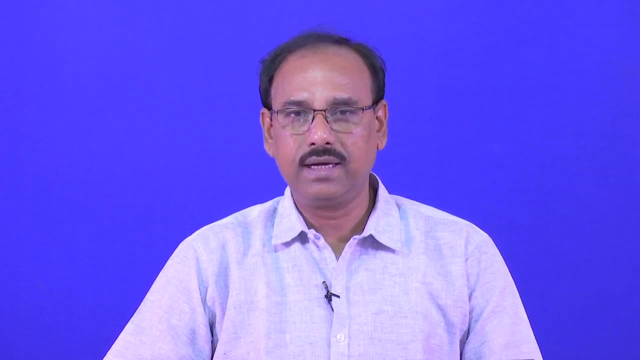 matrix, using the eigenvectors as rows in the transformation matrix And when you form this transformation matrix, as we have seen in your previous lecture, that the first row in the transformation matrix will be the eigenvector corresponding to the maximum eigenvalue and the last row in the transformation matrix will be the eigenvector corresponding to minimum. 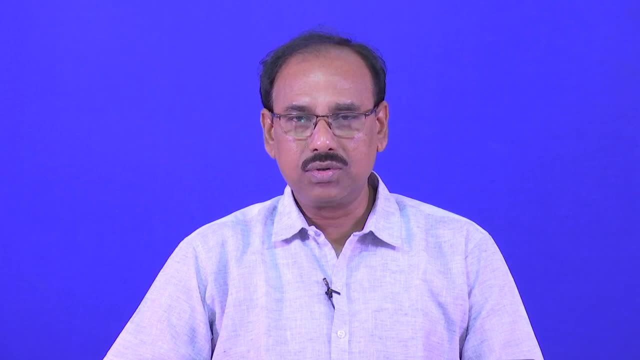 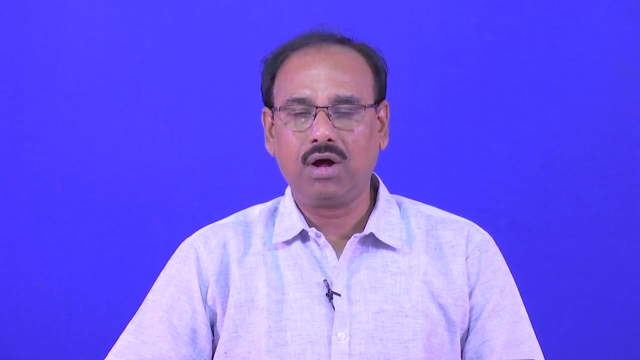 eigenvalue And in between all the rows are formed by eigenvectors, arranged in descending order of the corresponding eigenvalues. So now for transformation purpose, if we retain only few number of rows in the transformation matrix from the top, So we retain only one. 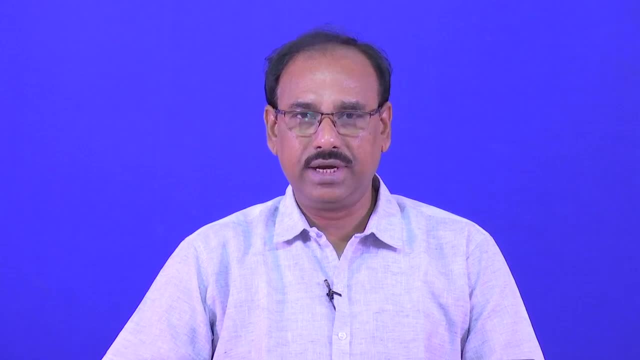 row. In that case, your d dimensional data is transformed into a one dimensional data. So, in that case, your d dimensional data is transformed into a one dimensional data, Which is nothing but projection onto the eigenvector, having my maximum eigenvalue. 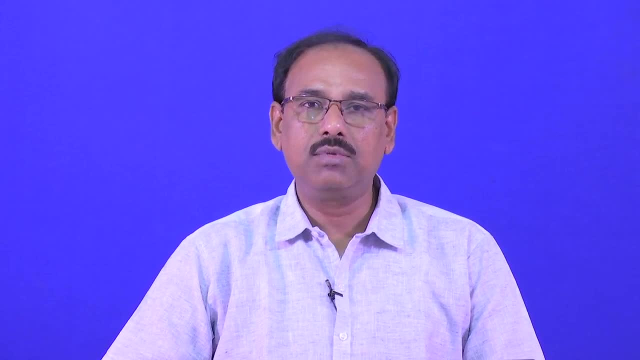 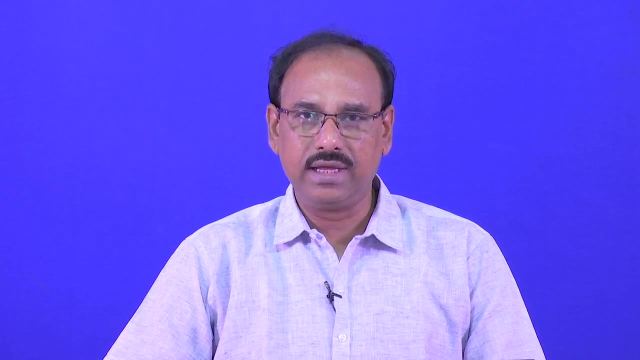 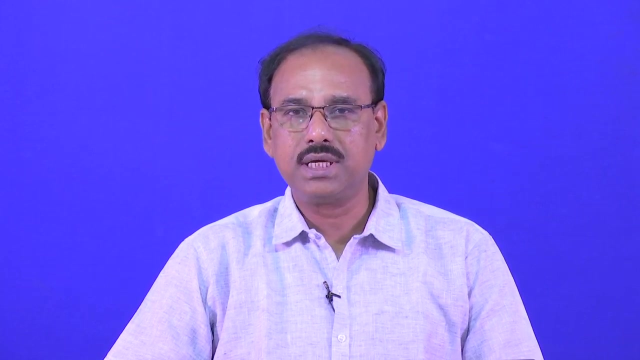 If we retain only two eigenvectors, then the d dimensional input data will be transformed into two dimensionalprinciple components in eigenspace. And we have also seen through reconstruction, with examples of reconstruction, that the power of such principle components. So we have seen with examples that even with 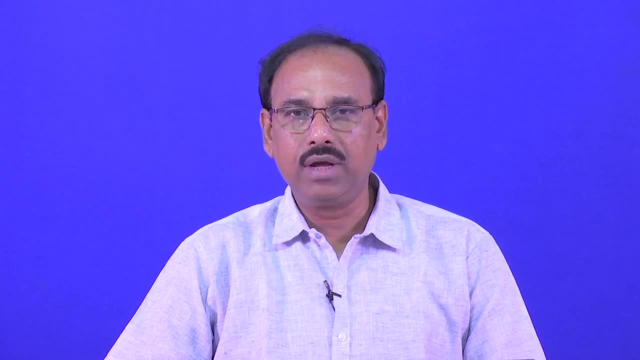 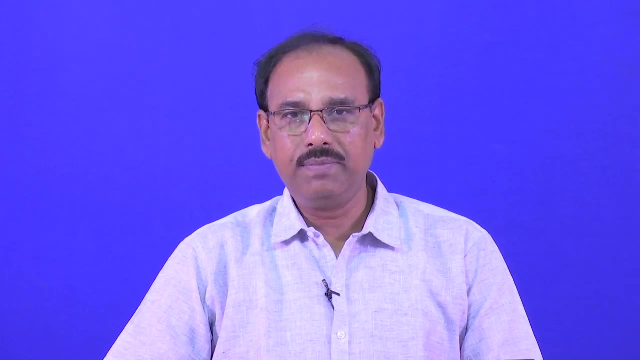 oneprinciple component, it is possible to reconstruct most of the information present in the input data. And there we have compared the principle component analysis PCA with autoencoders And we have seen that in case of autoencoder, if we do not impose any nonlinearity. 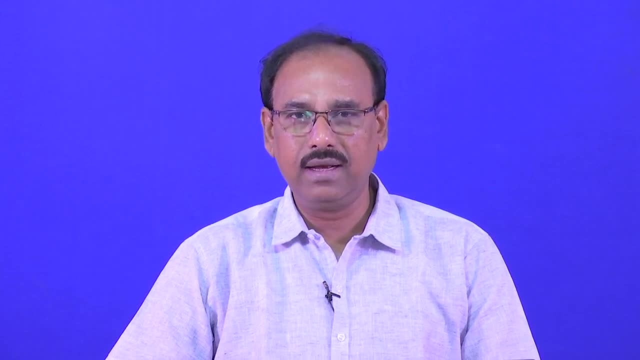 in the neural, in the neurons in the neural network, Then your principle components and the autoencoder outputs. they almost coincide. But we have also discussed that autoencoders are much more powerful than principle components because of the presence, because the neural neurons in the neural network are capable of imposing or implementing non-linear functions. 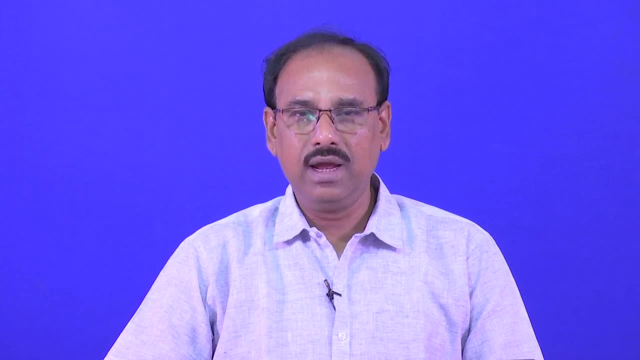 So as principle component analysis is a linear transformation from the input data to the input space, to the eigenspace, autoencoders can give you a non-linear transformation. So as, because autoencoders can give us non-linear transformation, we can even represent non-linear, 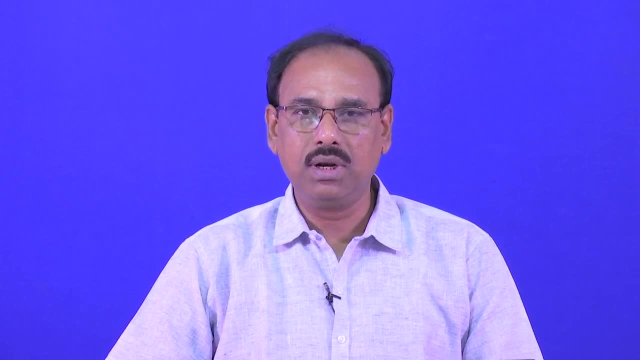 manifolds using the autoencoders, which is not possible using principle components. So you have seen that if we do not impose the nonlinearity, the nonlinearity in the neurons, or if the activation function of the neurons are linear, then autoencoder and principal component analysis. 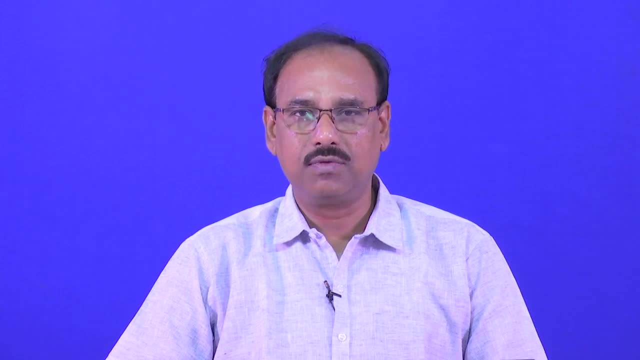 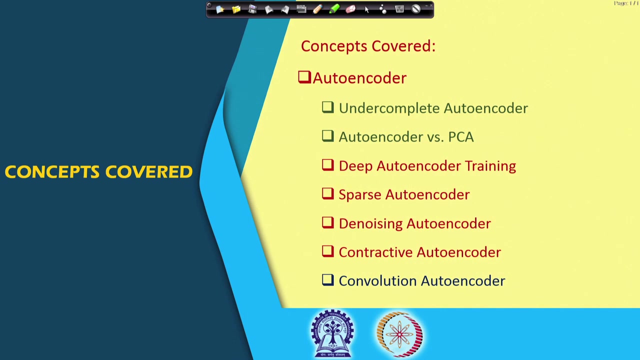 they become almost identical. However, because of the presence of nonlinearity, autoencoder gives us much better representation in lower dimensional space than in case of principal components. So that is what we have discussed in our previous lectures. So today, what we are going to discuss about is how do you train a deep 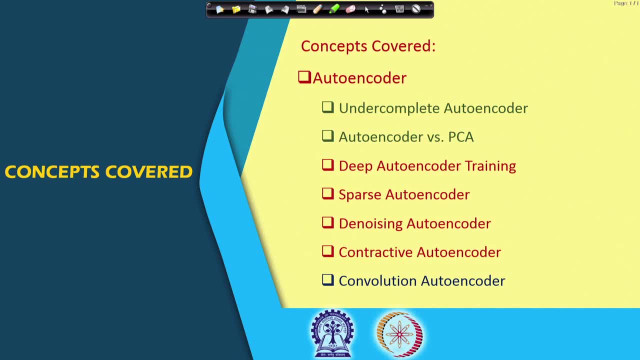 autoencoder. So we are talking about deep autoencoder training. then subsequently we will talk about other versions of autoencoders like sparse autoencoder, denoising autoencoder, contactive autoencoder and so on, And after few lectures we will also talk about convolution. 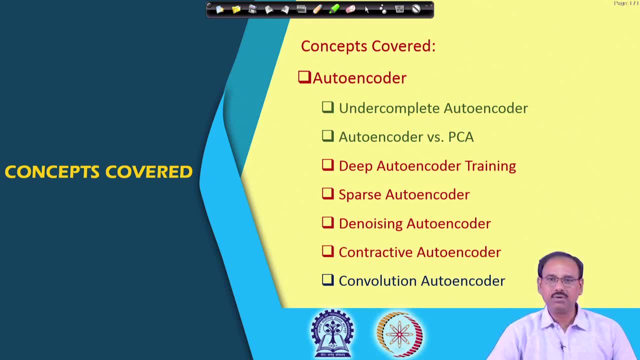 autoencoder, But I will come to that topic after we discuss about convolution and convolution neural network. So let us start with: how do we learn a deep autoencoder? So, as we told before that in case of deep autoencoder, and instead of having only one hidden layer, we have stacks. 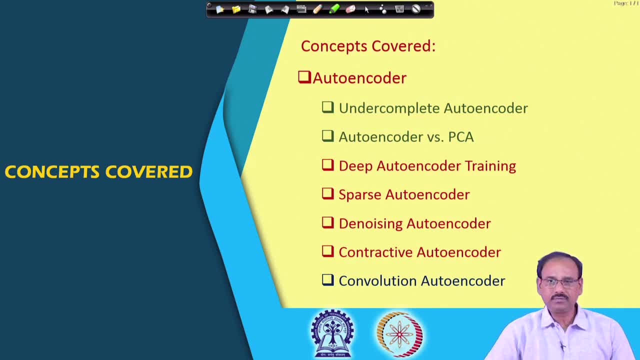 of hidden layers placed one after another. So that is what is necessary. So what is nothing but stacking of different autoencoder layers, and the depth of the network depends upon how many such autoencoder layers you have in your autoencoder neural network. 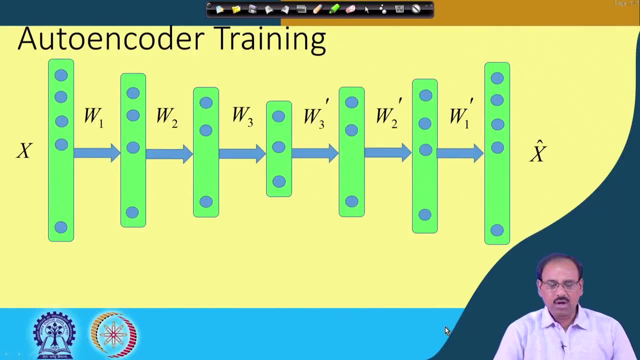 So a typical figure of a deep autoencoder is something like this: So here you find that we have our this input layer. So this is the layer which is input layer, input layer which is input layer. So you are feeding your input data x to this input layer. So 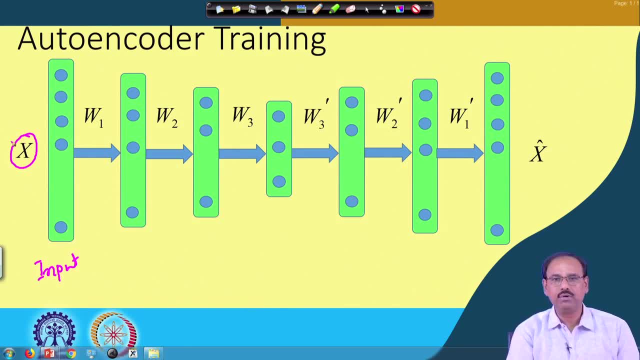 obviously the number of nodes in the input layer- we have also told that before- is same as the number of elements in vector x plus 1.. Why that additional one? Because we also want to incorporate the bias term in the same layer. So if the dimensionality of the input 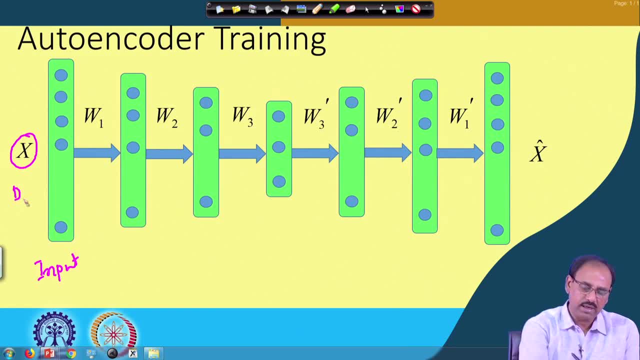 vector x is d, number of nodes in the input layer will be d plus 1.. So this is what we have discussed before, And then you find that we have a number of autoencoders, So I can call this one as, say, the first autoencoder, autoencoder 1, this: 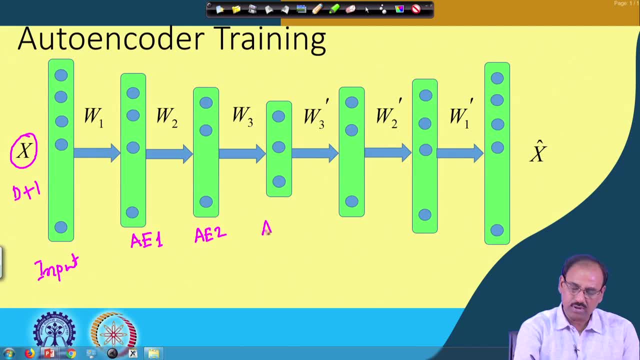 is the autoencoder 2, this is autoencoder 3, and so on, And here, in this configuration, I get the coded output. As you can see, this is the output, or the reduced dimensional representation, which is also known as latent spaced representation, at the output of autoencoder 3.. Of course, each of 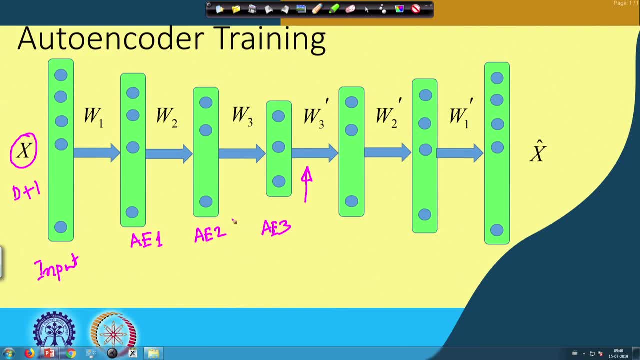 these autoencoders will give a reduced dimensional representation for the same input but at different levels. So output of autoencoder 1, what you get here is also a coded version of input vector x. Output of autoencoder 2 is also theicitized out that this without 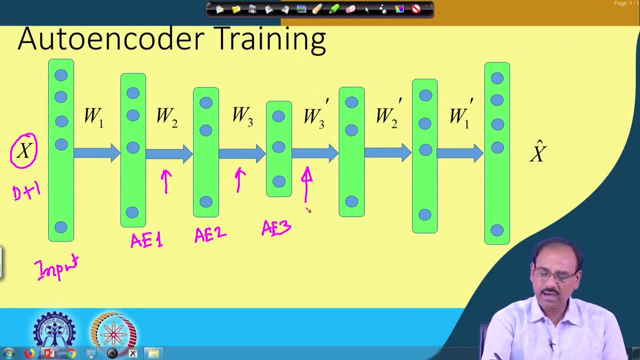 the input layer. So this will create a received recur flakes, also a coded version of input vector x. here. this is also a coded version of the input vector x, right? So this is where we get maximal dimensionality reduction And once I have this coded output, the coded output is decoded by this decoding layers. 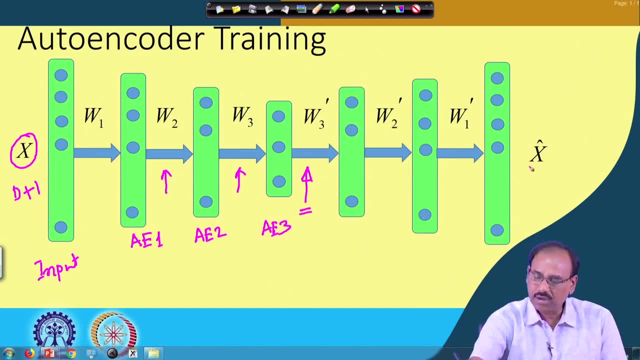 again, I have a number of decoding layers to get my reconstruction or the reconstructed signal x hat. So in case of autoencoder, what we said is we try to reduce the error between x and x hat or the loss function. in this case is L x- x hat, which we have also. 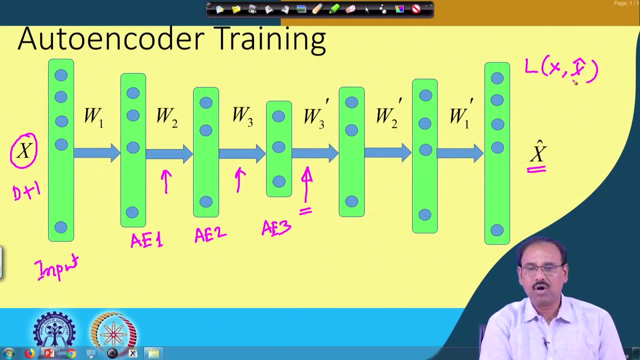 said that the loss function that can be defined is sum of squared error. that is what is the error in the construction of x hat when you compare that with input x, And so this is what we are trying to do. So training of the autoencoder or deep autoencoder will try to reduce this error at the sum of. 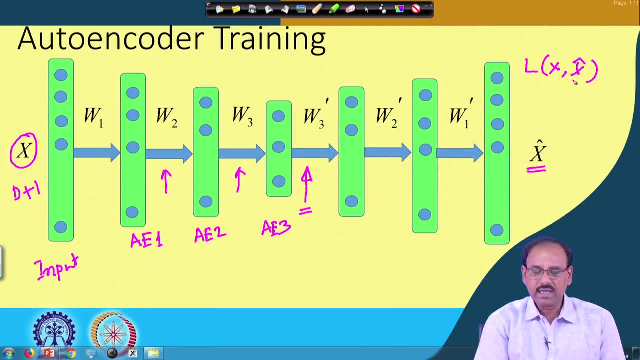 squared error to a minimum value. So you find that in case of autoencoder, we have also said before that I have an encoding part. So this is a portion which is encoding And this is a part of the autoencoder which is decoding. So I have an encoding portion. 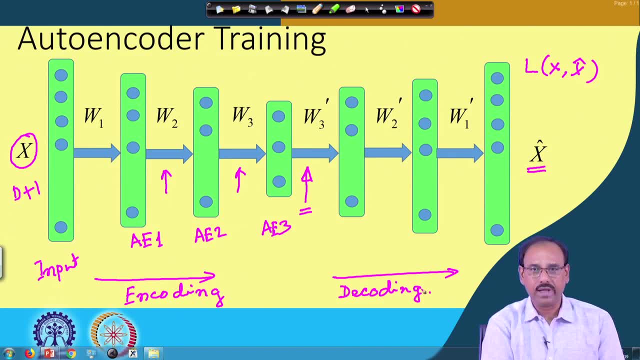 function and I have a decoding portion and these two taken together forms an autoencoder And the depth or the number of layers that you have auto, that you have within this one autoencoder, that tells you that what is the power of the autoencoder. ok, 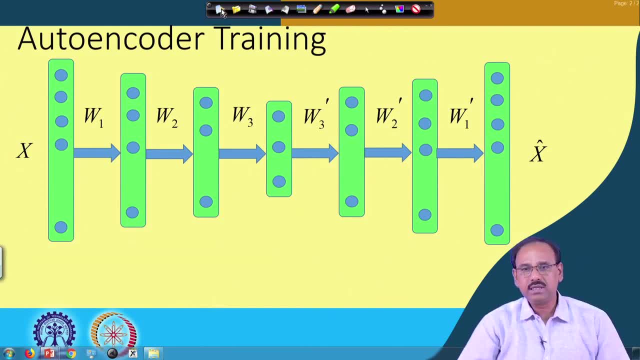 So, given this, that, as we said, that for training such autoencoder, I want to minimize the loss or minimize the error between the input vector x and the reconstructed vector x hat. So what I want, ideally, is the reconstructed x hat should be identical with my input vector. 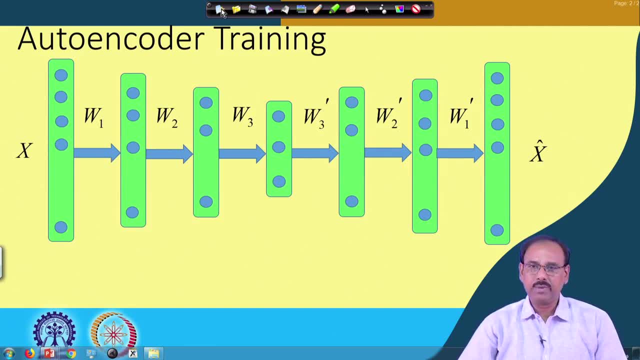 x, And that has to be done using the back propagation learning algorithm that we have talked about earlier. Now you find that the number of weight vectors or number of weight matrices. So that is the number of weight vectors or number of weight matrices, that 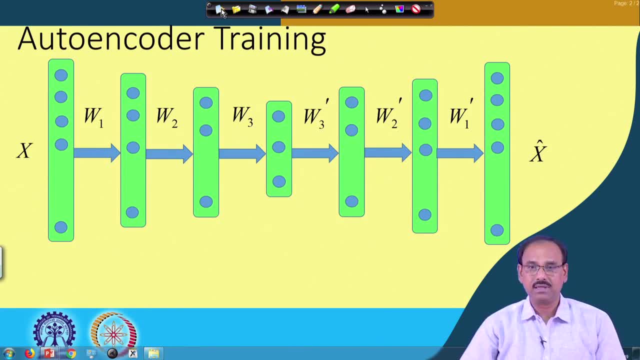 you have to determine by training of the autoencoder is tremendous. So I have weightmatrix W 1, I have weightmatrix W 2, I have weightmatrix W 3.. On the encoder side, on the decoder side, I have weightmatrix W 3 hash, W 2 hash and W 1 hash. And the number of weight matrices 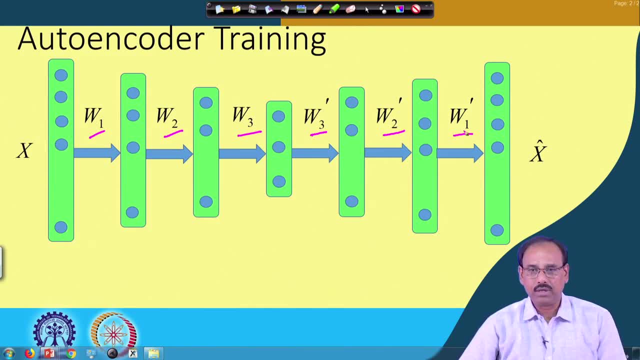 will go on increasing with the depth of the autoencoder. That is, the deeper the network is, the number of such weight matrices will go on increasing. So if I try to train this entire autoencoder end to end, that is, given the full autoencoder architecture I have- 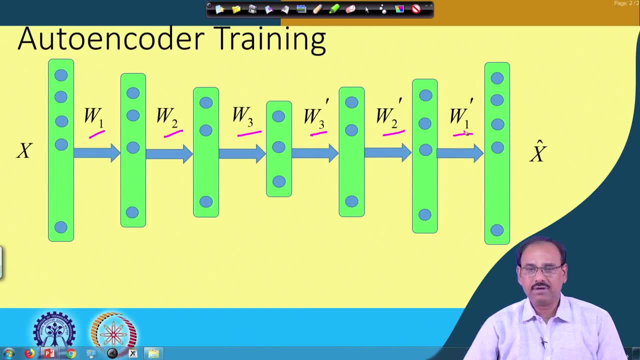 the state of training vectors given to the input. I have x, xhat as the output and by reducing the error between the input and the output, that is given to the input. So this is the between x and x hat. if I try totrain this autoencoder then I have to deal with so many. 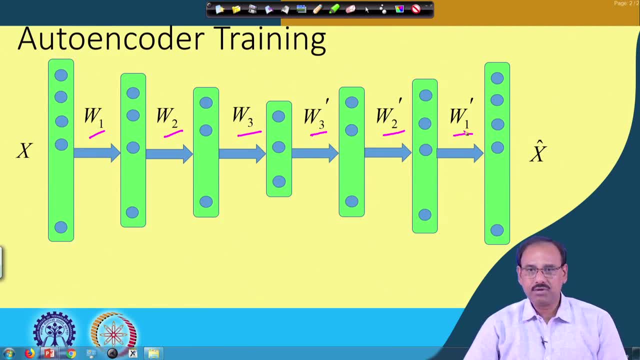 weight matrices simultaneously and that leads to a problem. One is obviously the memory problem that I have to save so many weight elements into into the memory. The other problems are that if the weights that you have is close to the solution weights, the convergence of. 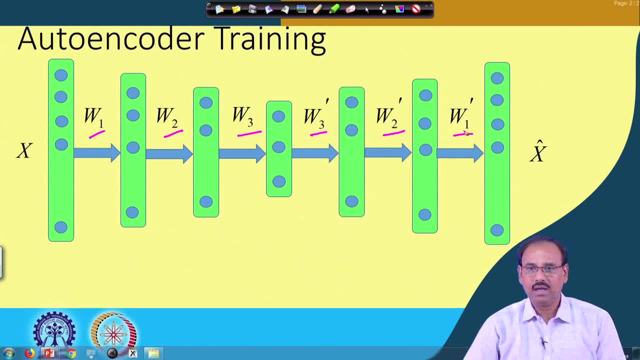 the learning algorithm is quite easy, But if the weight elements are too large, then finding a global minimum becomes the difficulty, And on the other hand, if the weight elements- because initially all of them are chosen at random, So if the weight elements becomes 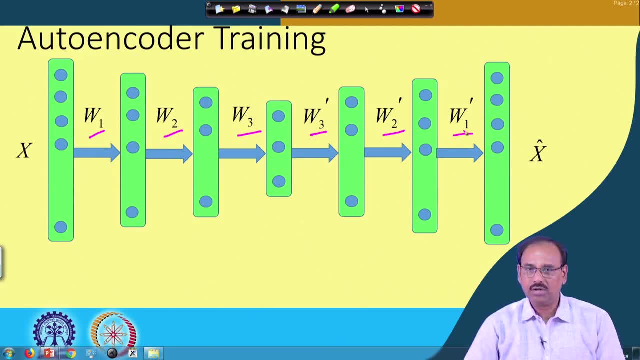 too low. in that case the convergence of the learning algorithm becomes very slow. So to avoid this problem, the kind of approach for training a deep autoencoder is called pre-training. Pre-training can be that you go for a stage called pre-training which will be finally refined with end to end training mechanism. 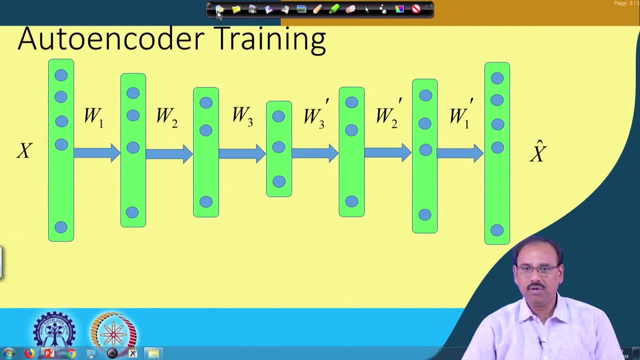 But before going for that, to reduce your complexity, you go for a pre-training, and this pre-training is done layer by layer. That means while pre-training you deal with lesser number of weight matrices. So let us see that how we how it is actually done. 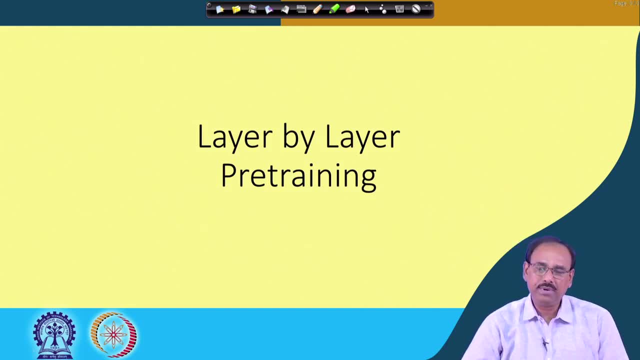 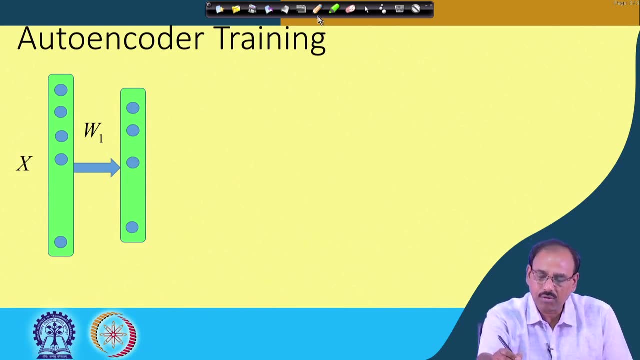 trip. So we are talking about the layer by layer pre training mechanism. So while doing this, you, I- take only one layer of autoencoder at a time. So, as before, I have this input layer where the input vector x is applied and I. 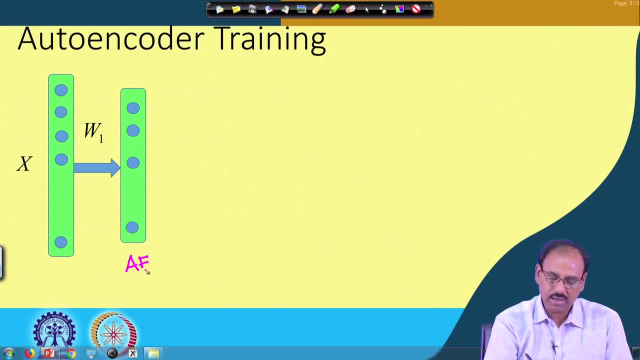 take initially only one auto encoder, say auto encoder layer one, And then I put a decoder which decodes the coded output from autoencoder 1. So because I have only one layer, this decoder output should besame as reconstructed X. So I call it X hat. and while training 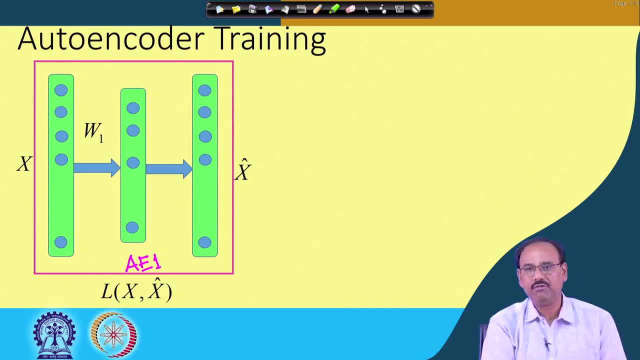 this first autoencoder, or while trying to determine what will be the value of W 1,, you go for back propagation and this back propagation will try to minimize the error between X and X hash, X and X hat and while doing so it learns the weight vectors W 1.. 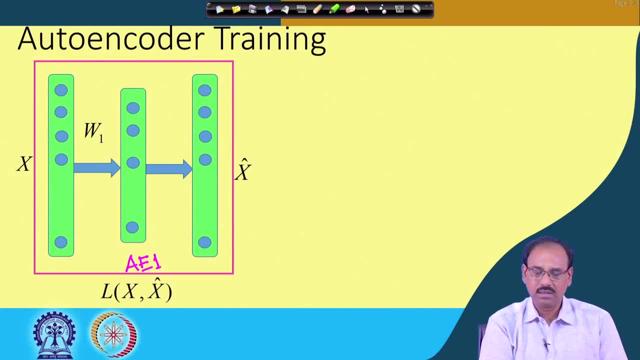 And once this weight vector W 1 is learned, then you discard the first level of decoder that we have used. And discarding this, now I put a second autoencoder Now, before that you find that, say, output of the autoencoder, which is an which encodes X, is say a latent space vector Z 1. So the 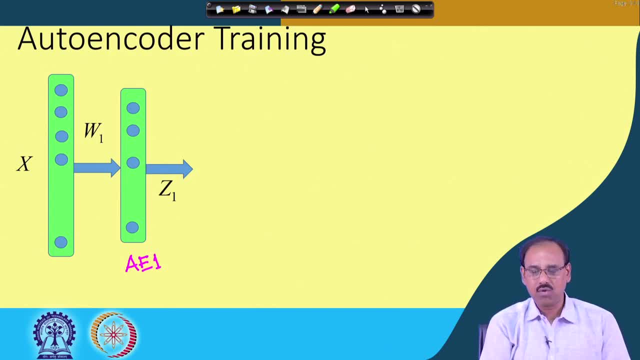 next level of autoencoder will try to encode this Z 1.. So I put the second autoencoder and let me call this second autoencoder as A e 1, A e 2, sorry. So this A e 2 will try to encode Z 1 and while doing so it will try to learn the weight W 2 or weight matrix W. 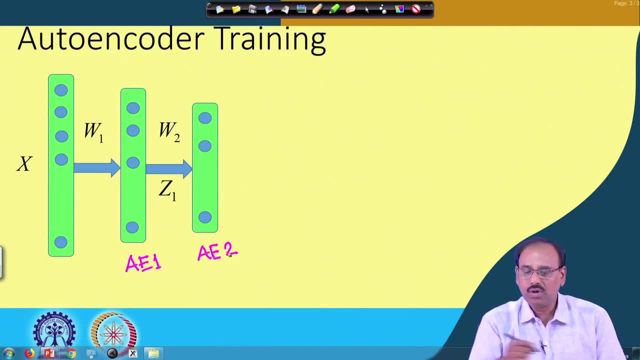 2, So to train A e 2. now what I do is I put another decoder. of course these decoders I am putting, they are all intermediate. finally, these decoders will not be there. So I put another decoder and this decoder tries to decode the output of autoencoder. 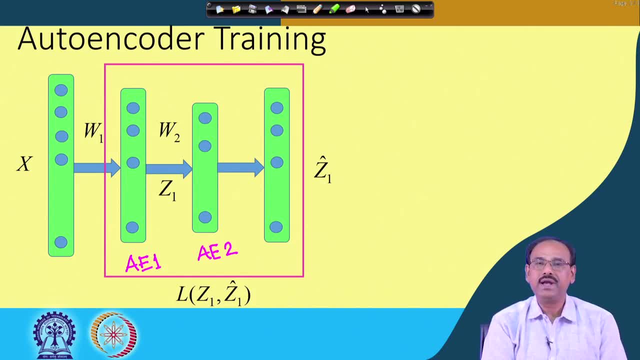 2. That means it will try to reconstruct Z 1, which is input to input to autoencoder 2 and I call this Z 1 hat. And for this learning, the back propagation learning, it will consider only the autoencoder 1, autoencoder 2 and the decoder that we have used And while training. 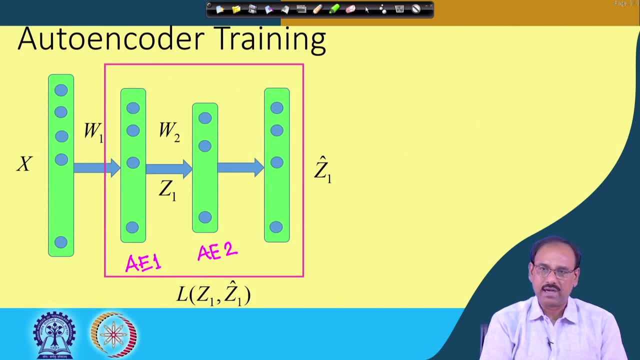 this. it will try to minimize the error between Z 1 and Z 1 and Z 1- hat, and once that training is complete, that learning is complete. what we have learnt is the weight matrix W 2.. And once weight matrix W 2 is learnt, you remove this second decoder that we have placed and 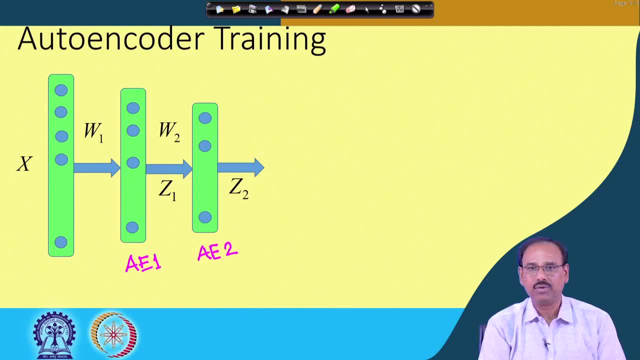 there the autoencoder 2, let me assume the output of the autoencoder 2 is Z, 2.. So the And after I got this I put the third autoencoder say A e 3. this is third autoencoder, A e 3.. 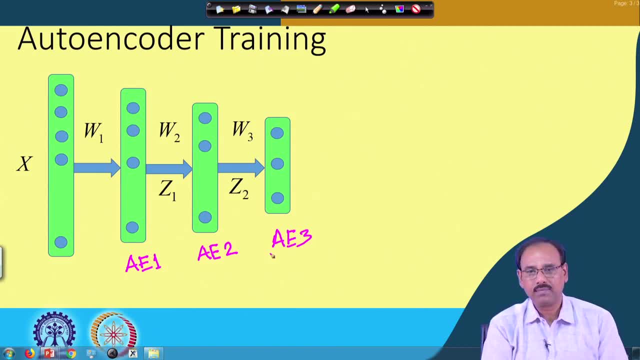 So now we have to train this third autoencoder. that means we have to find out that what are the weight, what is the weight matrix, W 3.. So again for training this, I put another decoder over here and this decoder will decode the output of autoencoder 3.. So you find: 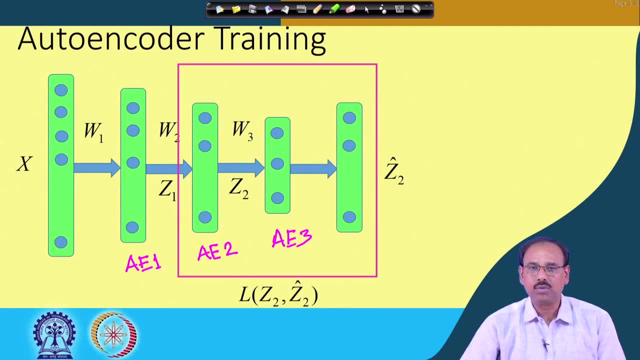 that the input to autoencoder 3 was Z 2, which was the output of autoencoder 2.. So this last decoder that we are talking about, this decoder will try to decode this Z 2 coded by autoencoder 3, to give you Z 2 hat. 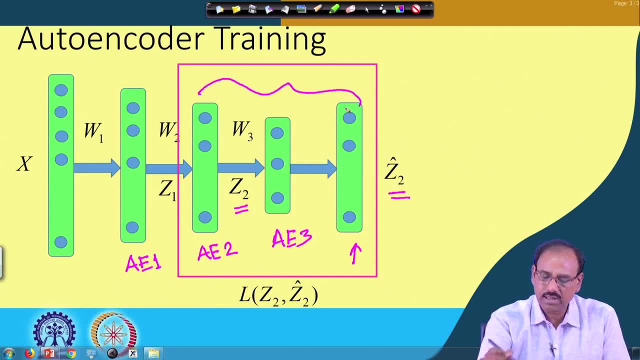 And for doing this, the layers which are involved is only these layers, and it will try to minimize the error or the loss function between Z 2 and Z 2 hat or L Z 2- Z 2 hat, and once that is trained, So you find that we have the pre trained values of W 1, W 2 and W 3.. And 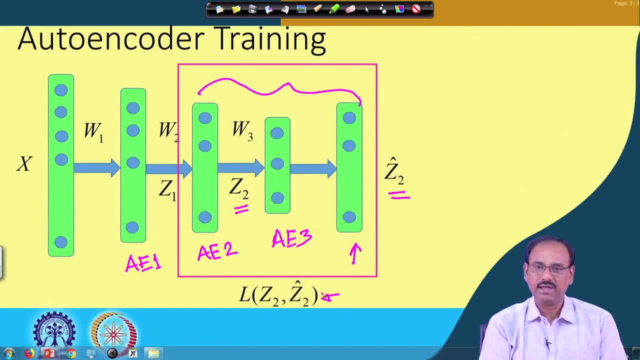 if I assume that this is the last autoencoder layer that we had in our deep training. So this is the autoencoder. then the next part comes is the decoder part. So to set the decoder. So what I have to do is I have to again remove this autoencoder. 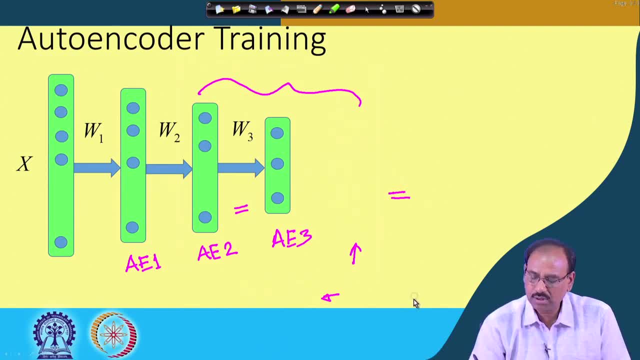 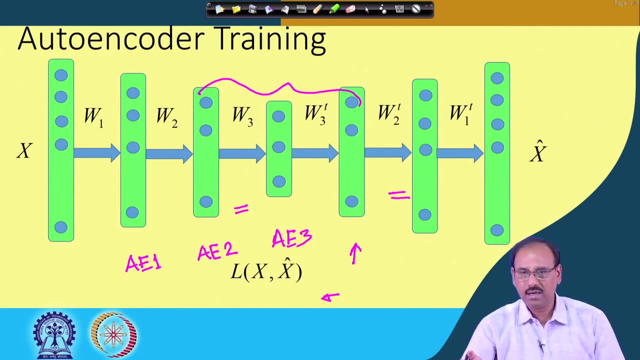 I have to have a decoder part. So the decoder that you put is this: by wrapping the encoder side and by taking the corresponding weights in the decoder side, you take the transposes Of the encoder weights, So this forms the total autoencoderor, the encoder decoder pair. 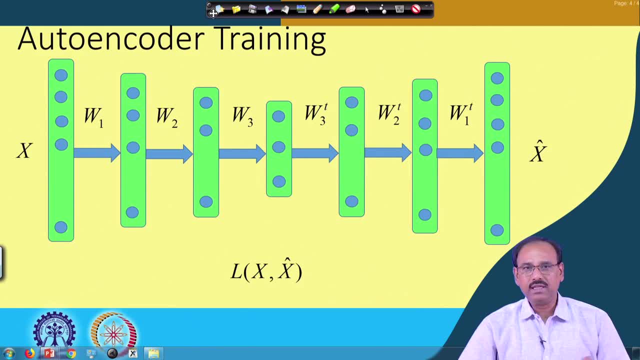 which forms the total autoencoder. So here you find that W 1,, W 2 and W 3. they were pre trained by using layer by layer mechanism, layer by layer learning mechanism. Now I have this decoder, also forming a full autoencoder. 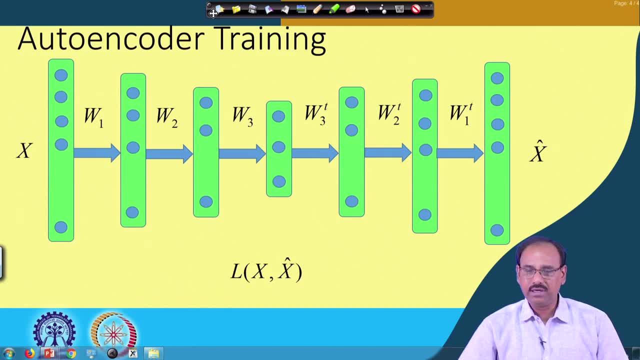 And now you go for fine tuning or finer training of the weight vectors. for that on the decoder side you initially assume that the weights are W 3 prime, W 2 prime and W 1 prime. Now you try to train this entire autoencoder. 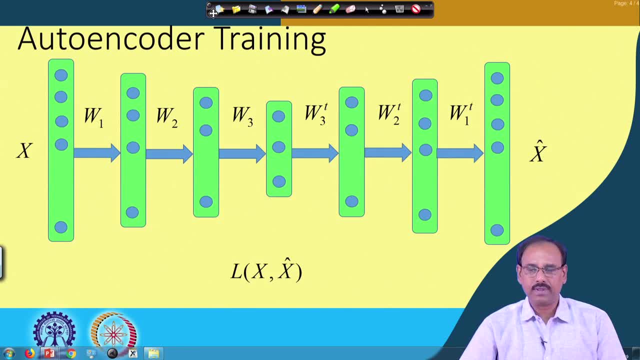 chain using end to end training mechanism, that is, you feed your training vector x to the input, So the output of the autoencoder becomes x hat, which is the reconstructed value of x, and by back propagation learning you try to minimize the loss function between x and 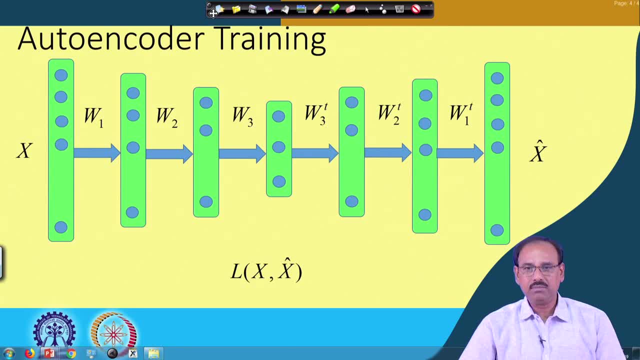 x hat, which is L x x hat. And here you find that because the encoder side was pre trained. So the values of the weight matrices W 1,, W 2,, W 3 are close to the actual values. So, as we are learning from a 가 nokta, we are considering the value above of x hat And as we are considering the value above of greatest value below of worst value above x hat, we are considering the value above of best value above x hat, And as we are considering, 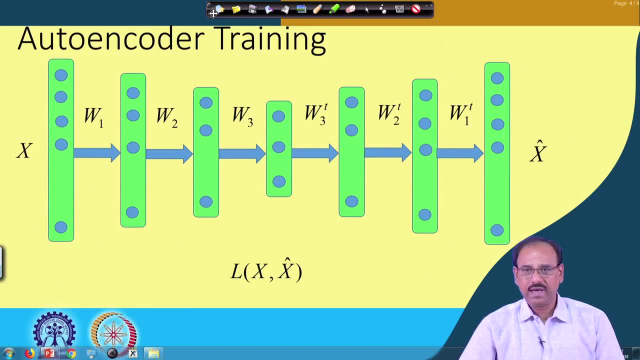 the value above of experienced modeling and And while you go for this end to end training. now we have set of values which are very close to the actual. the convergence of this training algorithm is much better than convergence of the algorithm if we try to train the entire network at a time. So this is what is layer. 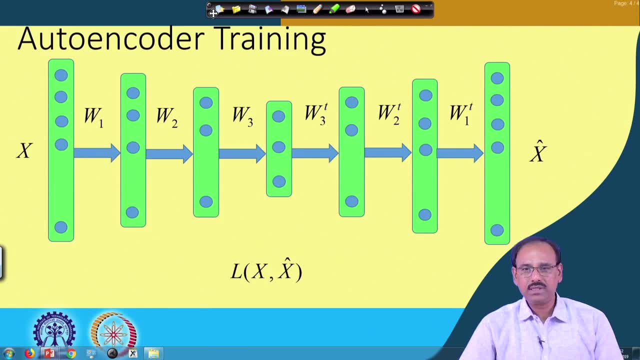 by layer pre-training. So what we have to do is, after the pre-training is complete, we have to introduce the decoder part, and then, for fine tuning of the pre-trained weights, I have to go for one or more iterations for end to end training, giving the input as x. 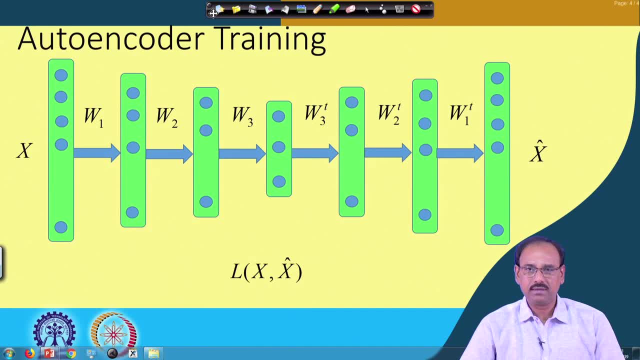 and the output encoder. output of the autoencoder x hat. try to reduce the error between x and x hat using the gradient descent or back propagation learning mechanism, So that will ensure the convergence to be faster and likely to attainthe global minimum of the loss function. So this is 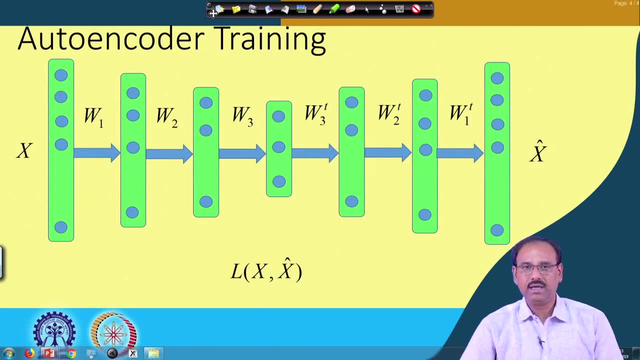 what isthe pre training, the layer by layer, pre training of autoencoder? Now suppose my autoencoder is trained. So what the autoencoder is giving me? giving an input X, the encoder side actually gives me, say, a function f of X. that is my encoding. 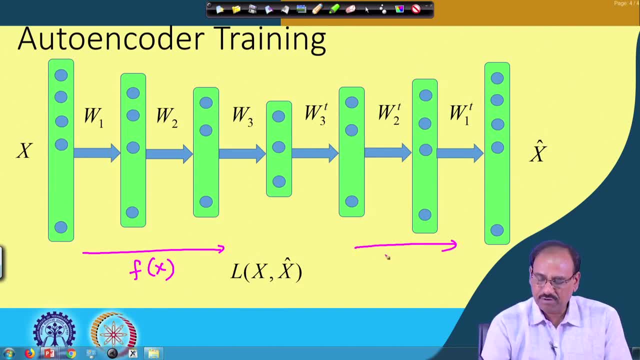 function, And so decoding, let me call it a function g. So this gives me decoding of f of X. So what is my x hat? X hat is nothing but g of f, X. So this is the decoding function. So this is the decoding function. So this is the decoding. 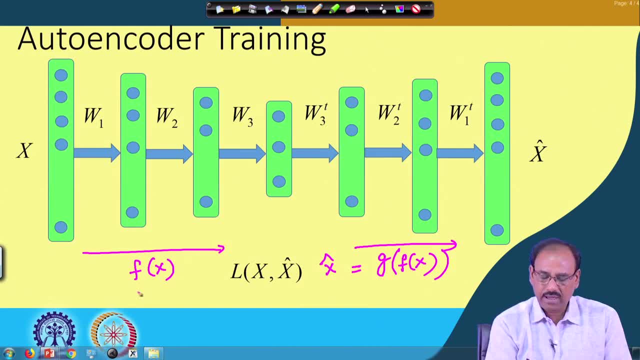 So the training mechanism try to minimize the error between f x and g of f x, and that is how you try to find that x and x at will be identical when the autoencoder is properly trained. ok, So, given this, as we said before, that we are not really interested in the reconstruction, 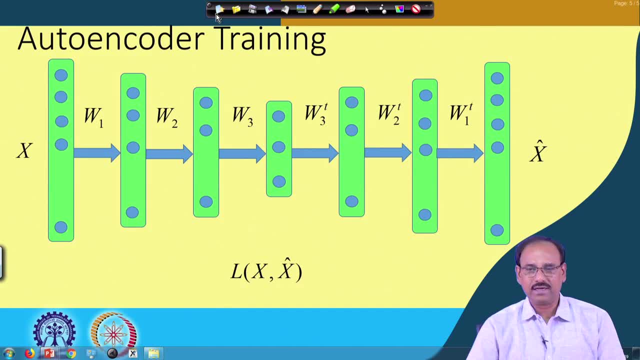 part. I have input x. what do I do with x at? that is not my aim, but my aim is actually the output of the autoencoder, That is, the latent space representation of the reduced space representation that I get from x and, as we said that, what I get at the output of 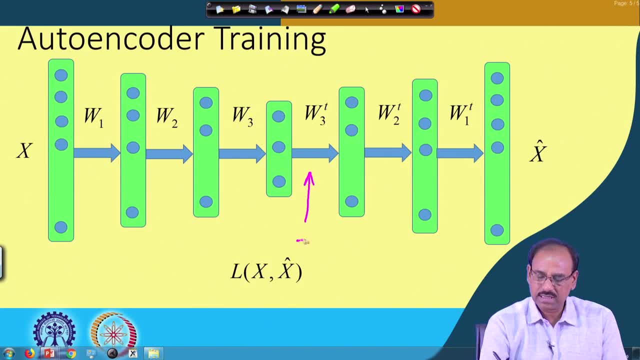 the autoencoder say: let me call this as output, vector h, which contains the salient features present in x, After discarding the redundancies or non salient features which are present in x. So h will contain the salient features, features and that is in the reduced dimension. So using H, how I can go for further applications? 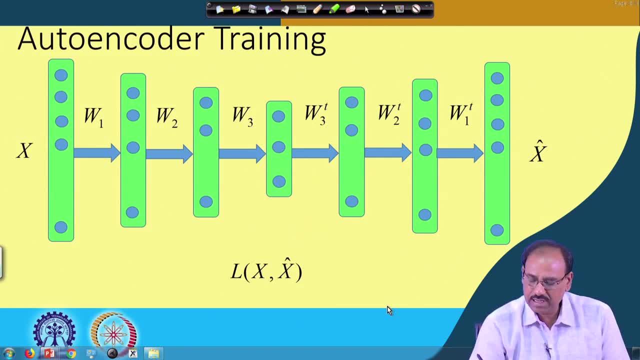 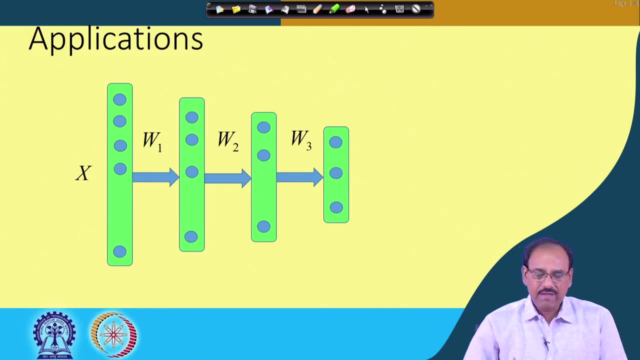 So one of the applications that can be- there are various applications. So one of the applications can be, say, classification. So what I have is I have input vector x, ah. So this input vector x, the output of the autoencoder, gives me H, and here this H can be fed to a classifier. 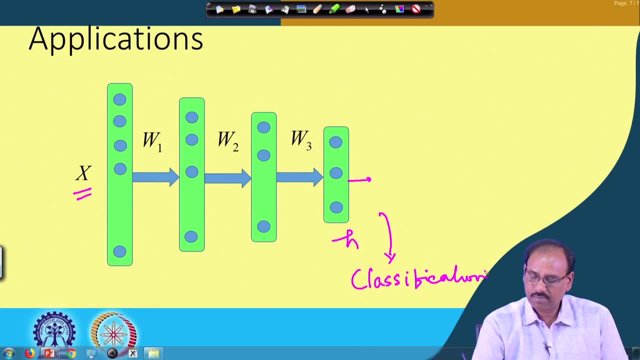 for classification. It is not necessarily that classifier. this classifier has to be a neural network. it can be any classifier, it can be a support vector machine, it can be a base classifier or whatever which we have discussed earlier. But let us assume that we have a neural network we have talked about. 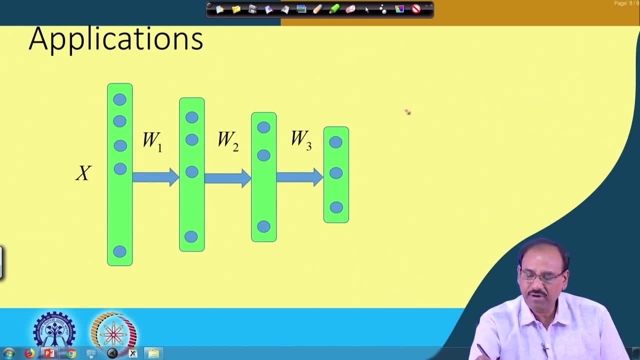 We have talked about multi-layer perceptron before, So I can feed a multi-layer perceptron, or MLP, over here. So the input to MLP is H and output of the MLP is the class identification of H or eventually the class identification of the input vector x. So now we find that 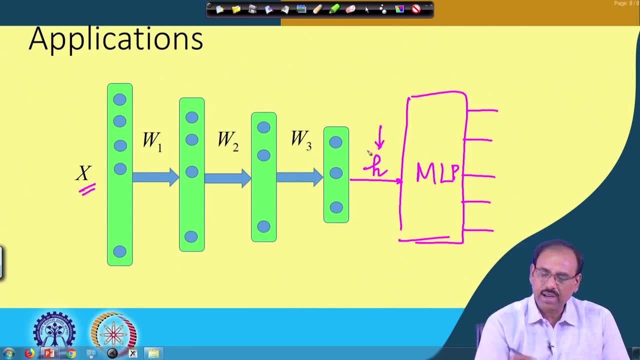 what the autoencoder does is. it gives a coded output H, H of x. it does not give you what isthe class belongingness of H or what is the class belongingness of x. So if for the training vectors the class belongingness of x is also known, that 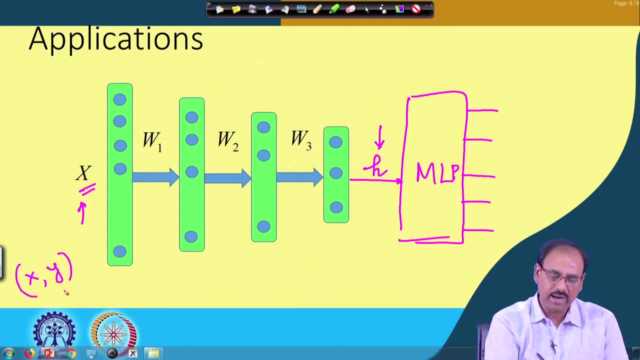 is the training. vectors are given in the form of x- y, where x isthe input vector and y is the class. Then again, I can go for an end to end training, fine, with finer refining of the weight matrices, W 1,, W 2,, W 3, and now this training, this back. 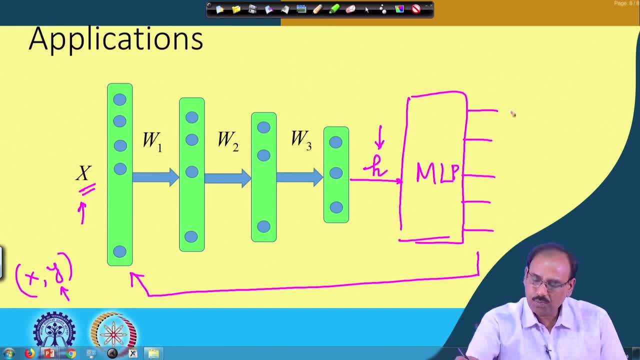 propagation training will consider the output of this MLP or will consider the loss function? with the output of the MLP, that also we have seen before, It can be cross entropy, it can be again sum of squared error. So the lossoutput error function, So the loss function can be defined, which is defined. 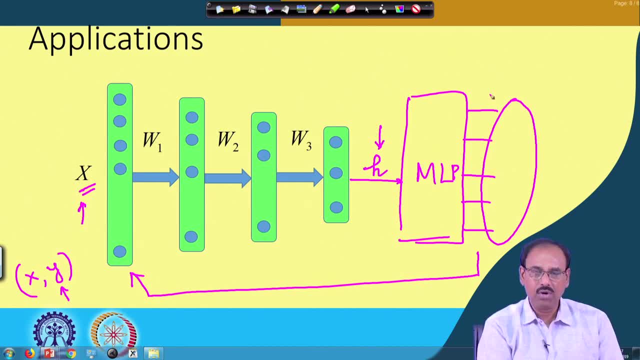 at the output of the MLP, depending upon whether the class say y hash, which is decided by this MLP taking this H, that matches with y or not. If it matches with y, then there is no error or no training required. if it does not match, then obviously we have to train this interneural. 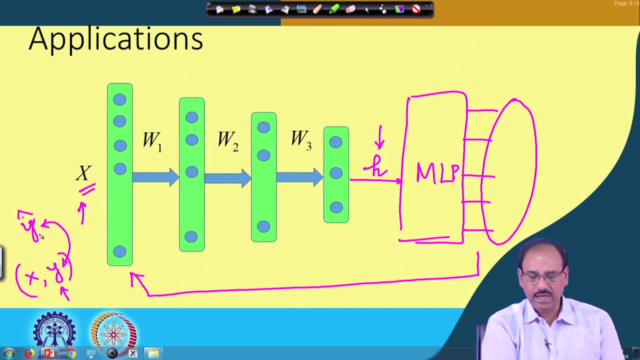 network with back propagation, learning, And during that time also this W 1 to W 3, this encoder, encoder weight matrices can be defined further. This is one of the application. The other application can be, even I can go for, say, pixel classification or segmentation operation of an input image. So for that, 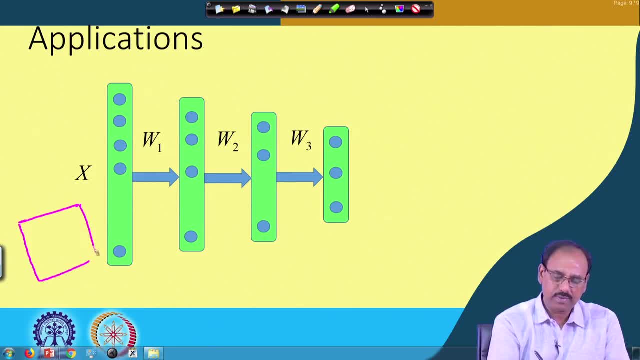 what I can do is suppose I have an image and input. you take various patches of this input image, convert that into a vector and feed that to the input And, as we have seen before, that output of the autoencoder will contain the salient features. 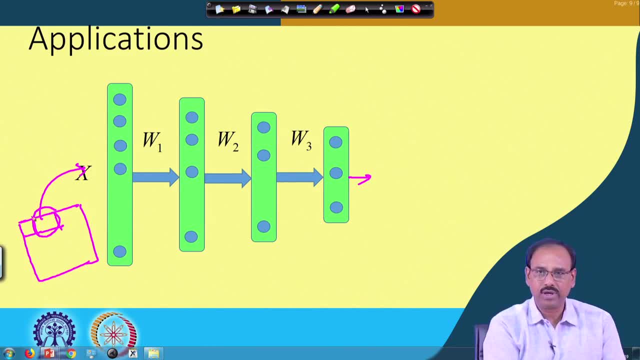 of each of these image blocks. that is what the autoencoder is doing. And then, at the output again, I put a classifier. What this classifier will do? It will put this input matrix, the input image or patch of the image, into one of the classes And if that class 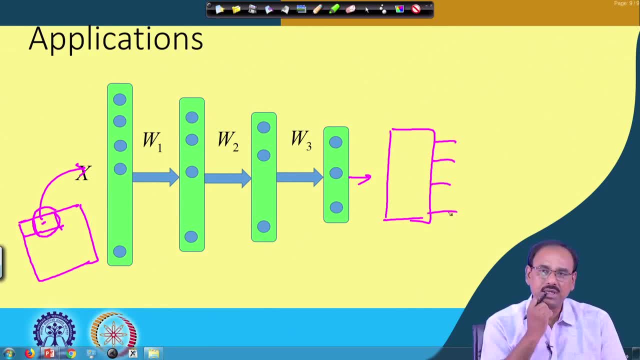 and using that again I can form an error function or a loss function and the autoencoder can again be trained using this loss function. And finally, once the autoencoder is trained again, now you feed an input image again, feed all the different blocks of the input image. 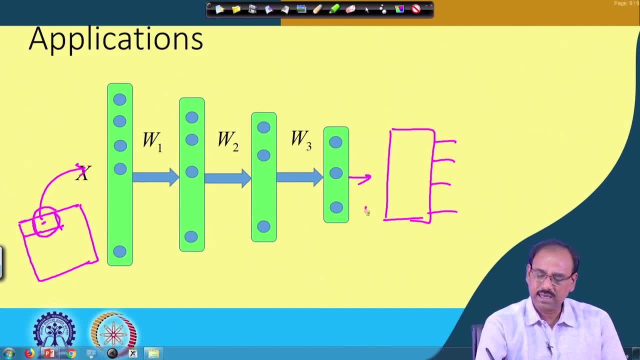 to this autoencoder. the autoencoder will give a salient or the latent space representation of each of the blocks, and the blocks can be classified by this trainedMLP, So thereby I can classify each and every block in the image, which is nothing but a segmentation. 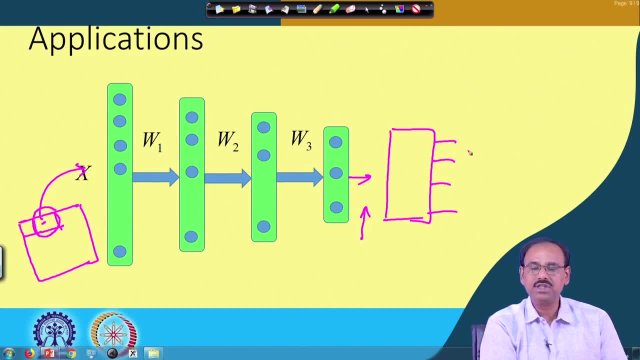 operation. I can also consider this to be a pixel by pixel classification, orthe semantic segmentation of the input image, And for that what I can do is given an patch in the image. whatever representation I am getting at the output, I can consider that this is the salient features of the central. 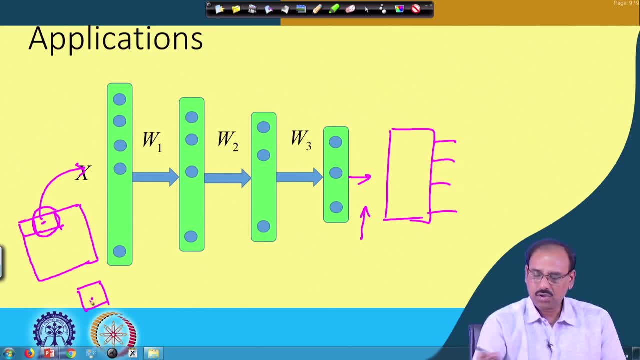 pixel of this patch. So this is my central pixel. So this classifier output basically classifies the central pixel. So as I take different blocks of the image and pass it through the autoencoder and classifiedchain, Then the classifier output will classify each and every pixel which is the center of the 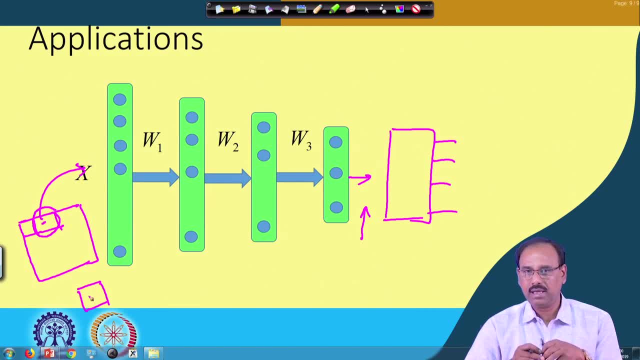 block. So it will classify each and every pixel within the image to different classes. So the classification of pixels to different classes is nothing but segmentation of the input image. So the input image, or the pixels in the scene of the input image, are now classified. 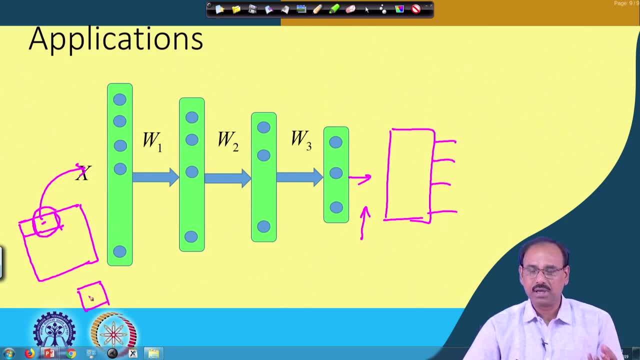 into different class And all the pixels belonging to the same class that forms the a particular segment. So today what we have discussed is that: how you can train an autoencoder. we have talked about layer by layer training of the autoencoder, And once the autoencoder 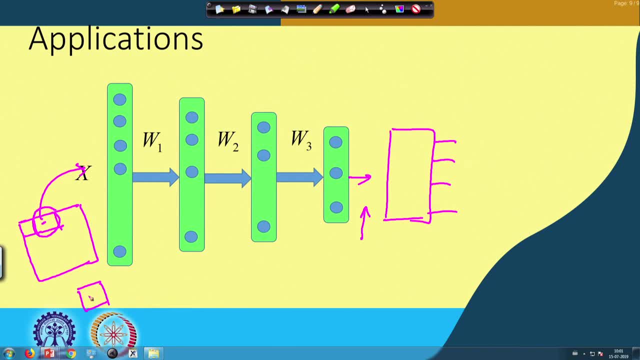 is trained what can be possible applications of such autoencoder. So we will stop here today, Thank you.